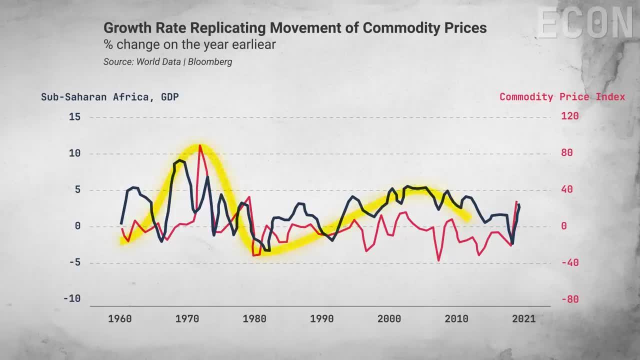 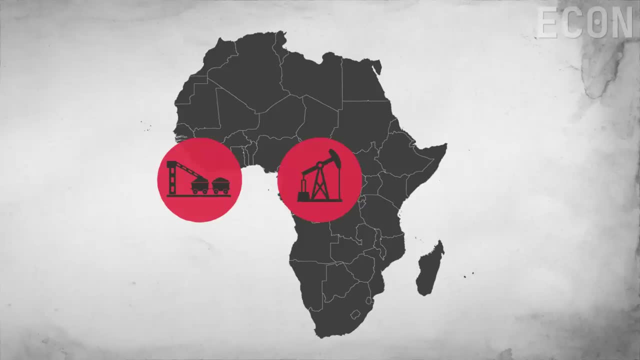 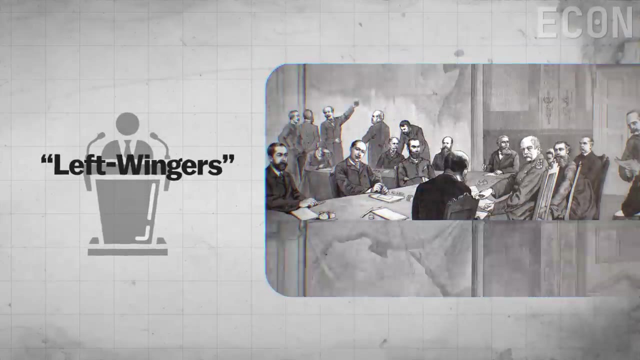 growth was good. when prices dipped, the continent economy suffered as well. even though africa is home to a third of the planet's mineral reserves, a tenth of the oil and two-thirds of the diamonds, it is still the poorest continent on earth. many left-wingers argue that africa is poor because 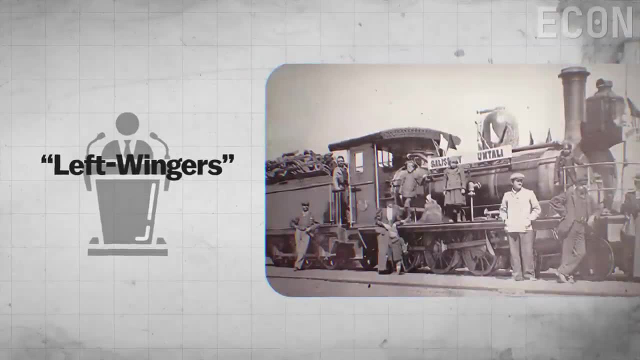 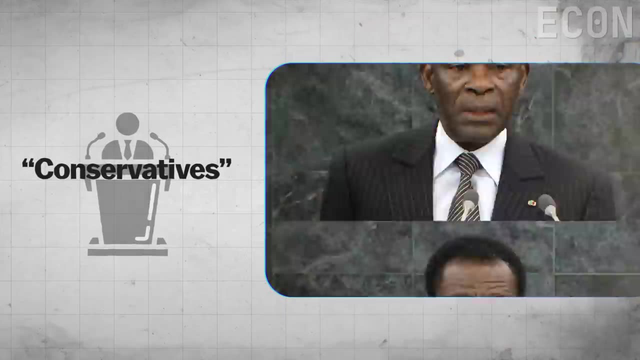 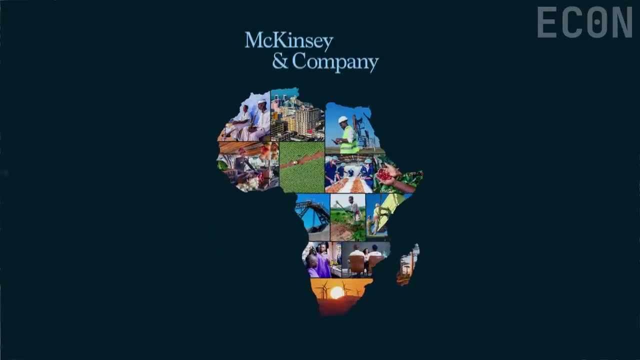 its former colonial powers want to keep it that way, not because of the choices its leaders are making. many conservatives, on the other hand, sweepingly say that corruption or bad governance are to blame, without taking account of the obstacles many african countries face. however, according to mckinsey and company research, africa is outperforming many expectations and transforming. 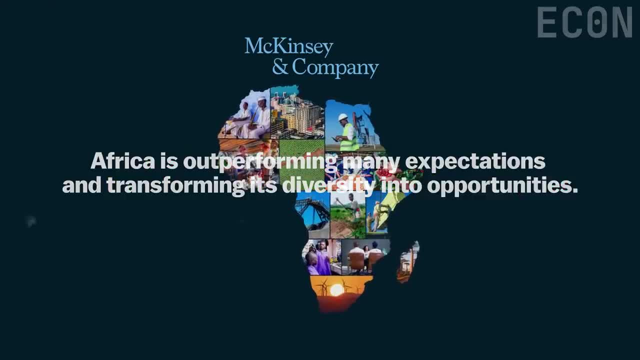 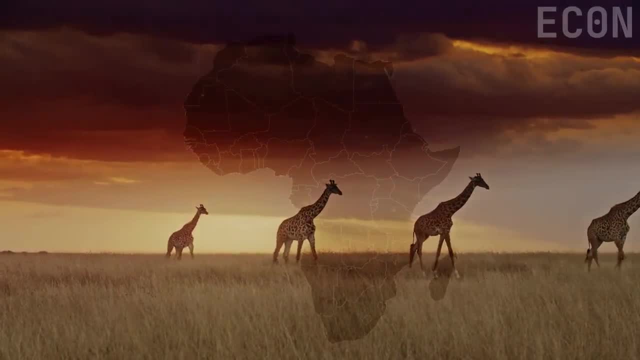 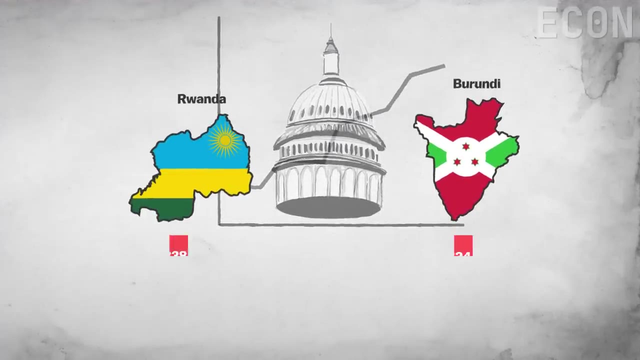 its diversity into opportunities. so let's delve into the details of how similar countries have taken diverse paths, offering valuable lessons to be learned. the first lesson, about the importance of simply having a state that works, comes from rwanda and burundi. both countries are small, landlocked and 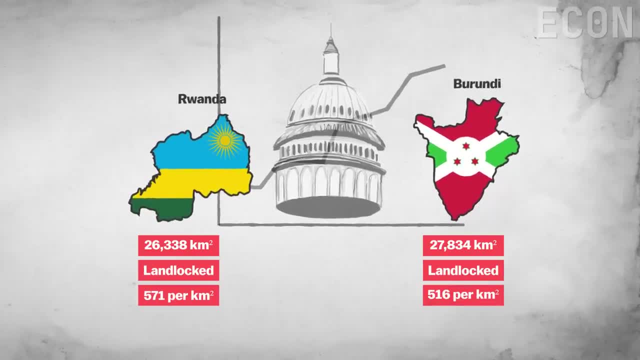 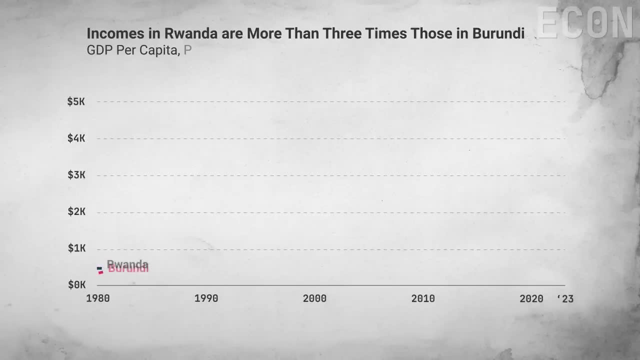 densely populated. since gaining independence, both nations have experienced genocides against their tutsi minorities by their hutu majorities. in the early 1990s, burundi had an income almost similar to that of rwanda. however, since then, incomes in rwanda have more than tripled. 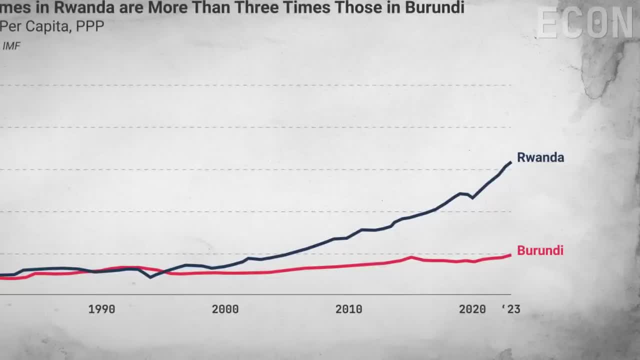 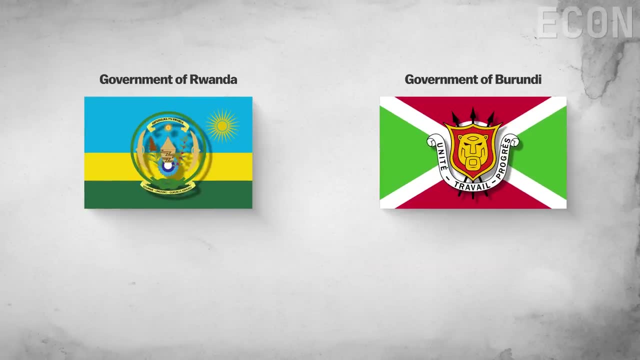 whereas those in burundi have fallen, resulting in it becoming the world's poorest country. one significant difference between the two lies in their governance. although neither country is democratic, rwanda has a functional government and low corruption, whereas burundi witnessed large scale political strife and various coup attempts. the ibrahim index of african governance, which looks 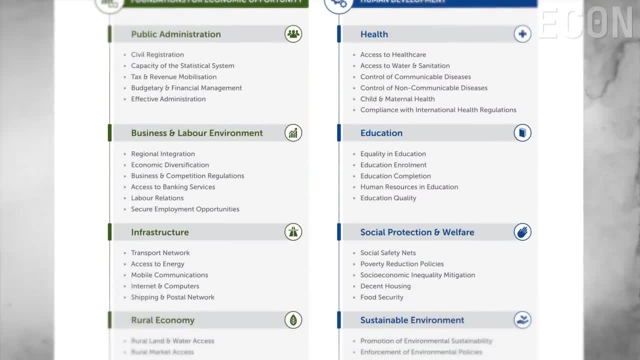 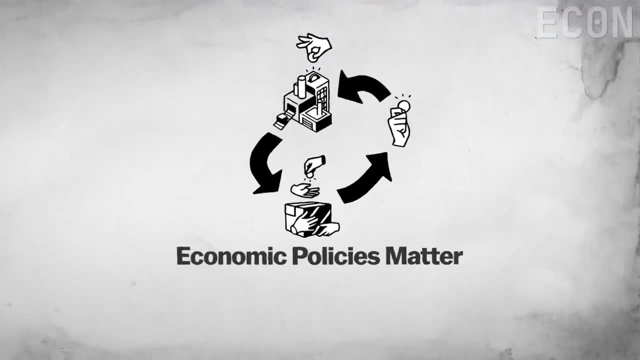 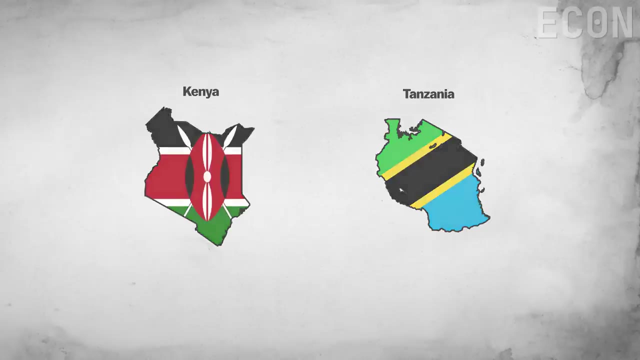 including the rule of law, infrastructure and sanitation, ranks Rwanda 12th, while Burundi is placed 43rd. The second is that economic policies matter. Upon gaining independence in the early 1960s, Kenya and Tanzania had similar economies, both dependent on farming, with almost identical 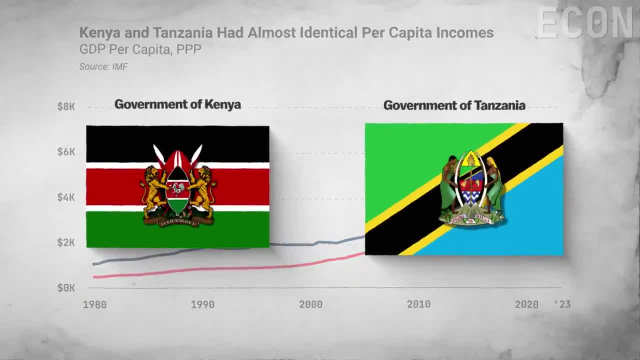 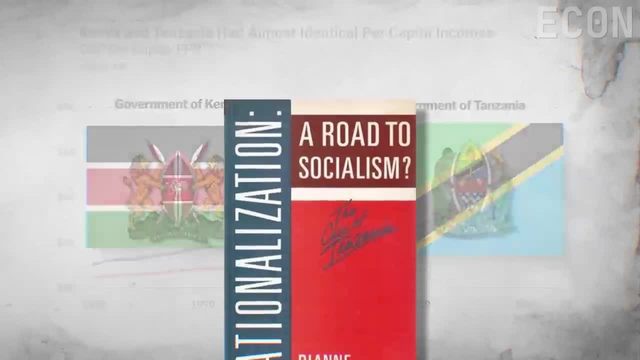 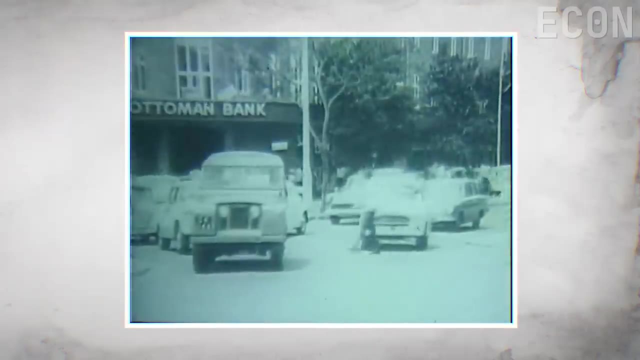 per capita incomes. Both initially suppressed democracy to run authoritarian, one-party states, but they chose very different economic models. Tanzania nationalised big companies and forced people onto collective farms in the name of African socialism, while Kenya embraced free markets, which encouraged investment and implemented several regulatory reforms to 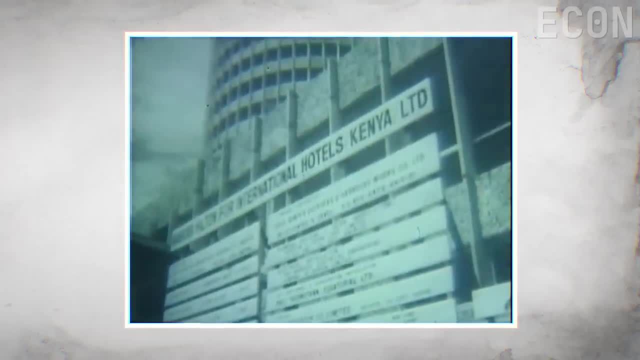 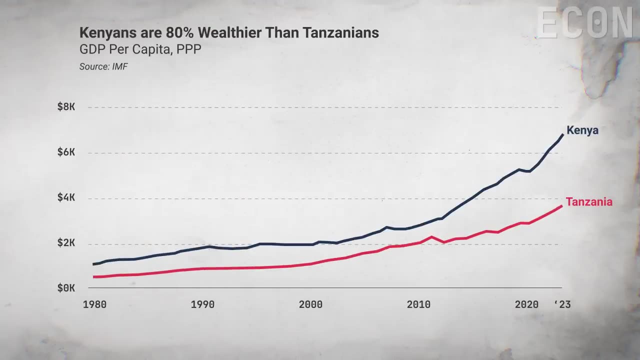 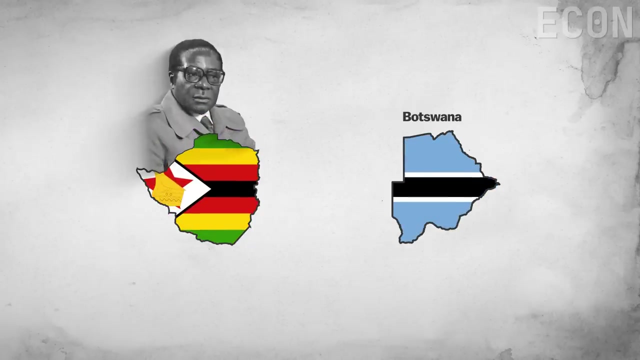 streamline foreign and local investments, including the establishment of an export processing zone. As a result, Kenyans are now 80% wealthier than Tanzanians. Zimbabwe and Botswana further react. Both the countries are led by very different, temperamental political leaders In the early 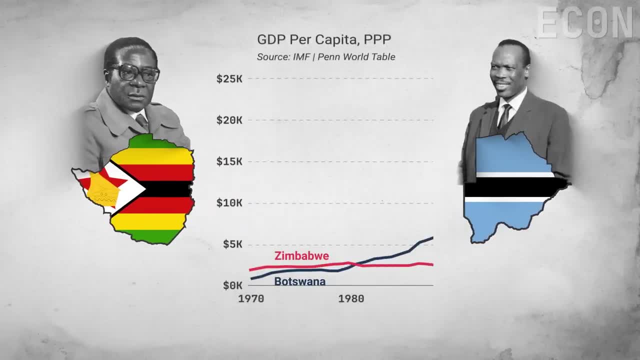 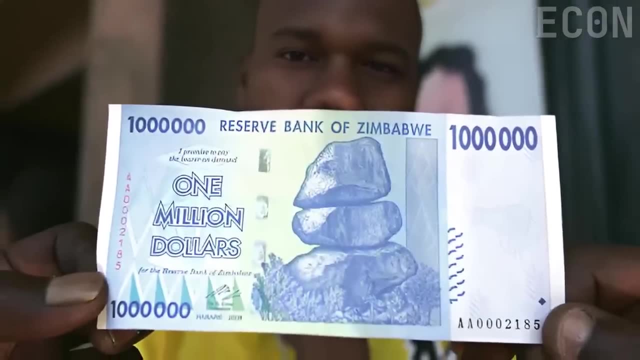 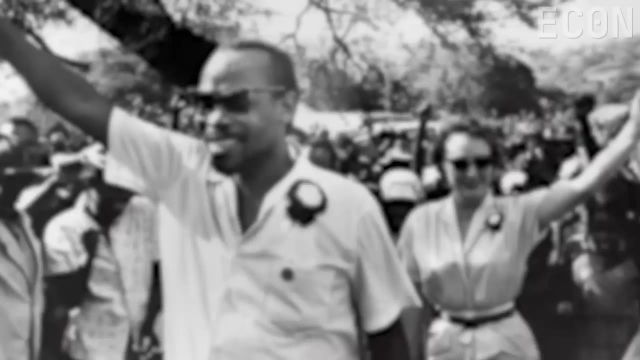 1980s, Zimbabwe was richer than Botswana. However, Zimbabwe's second president, Robert Mugabe, destroyed its economy through careless printing of banknotes, stealing farms for his cronies and authoritarian rule, Whereas Botswana's first president, Serece Kama, embarked on an 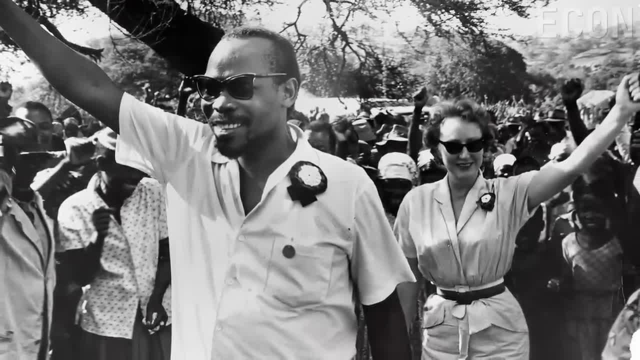 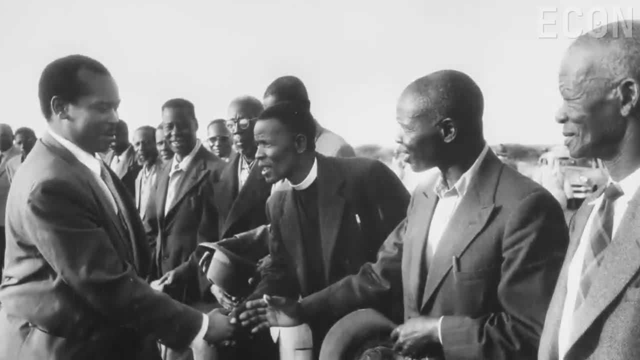 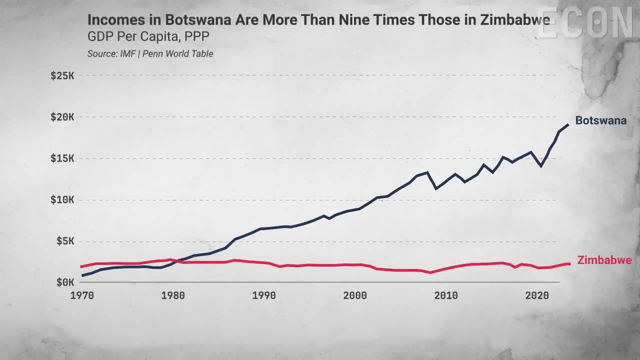 ambitious economic agenda aimed at reshaping the nation into an export-driven economy centred around beef, copper and diamonds. Kama implemented stringent measures to combat corruption. Consequently, Botswana now enjoys a wealth that is nine times greater than that of Zimbabwe. 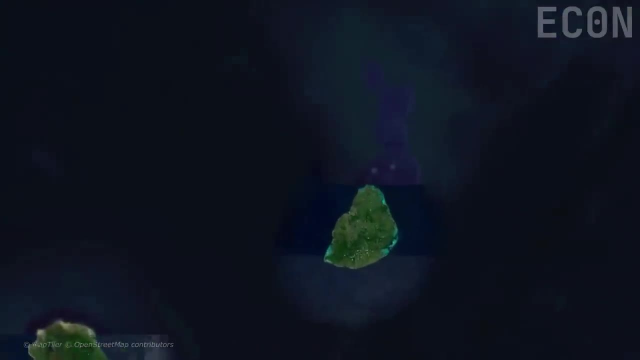 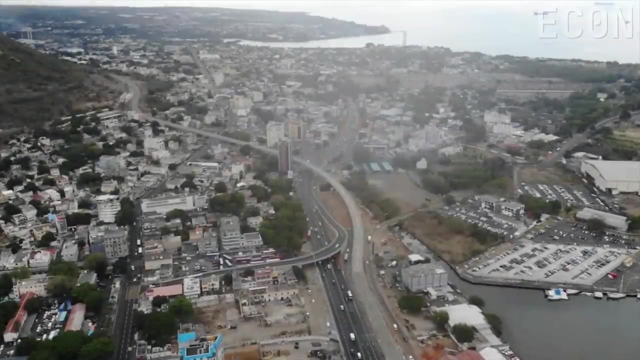 Let's take a look at Africa's most successful economy, Mauritius, With one of the highest GDP per capita and HDI scores. it serves as a remarkable example of how countries with sound policies and robust institutions can enter a virtuous cycle of development. This 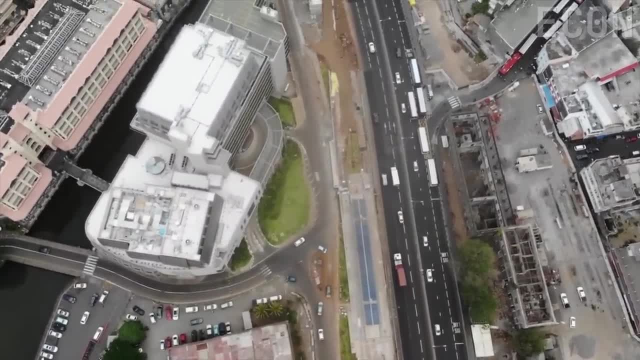 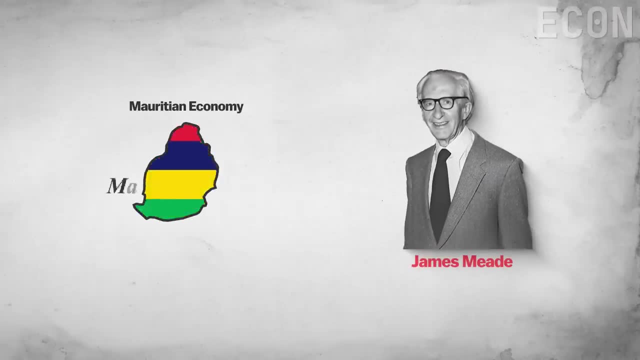 small island economy has been a historical evidence against the pessimistic projections made by Nobel laureate James Mead. Mead regarded the Mauritian economy as a case of the Malthusian Trap, predicting poor developmental prospects due to its heavy reliance on a sugar-based. 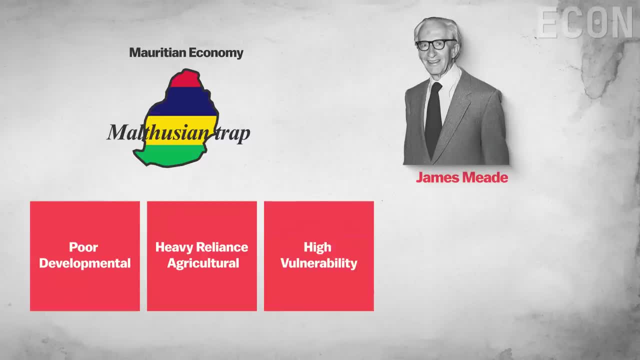 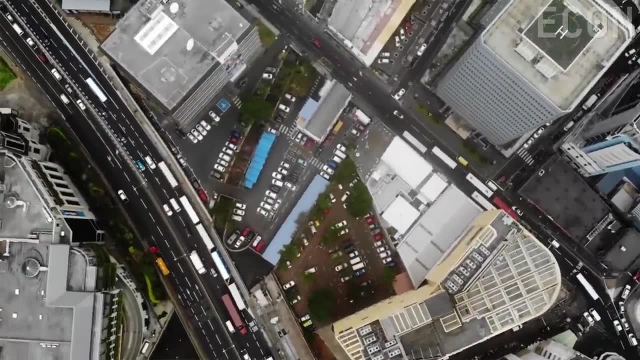 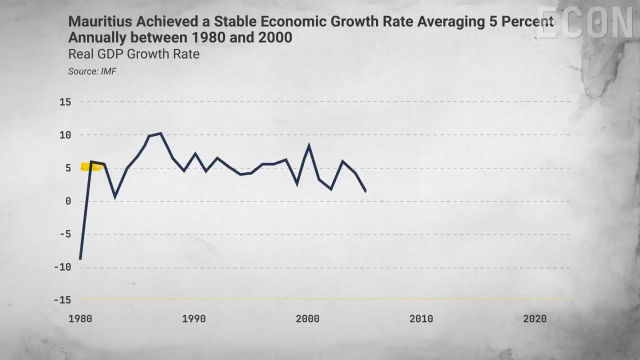 agricultural sector, high vulnerability to trade shocks, rapid population growth and rising ethical tensions. Yet, in addition to maintaining national stability and social cohesion, the island economy has sustained a high economic growth. The island economy has a stable economic growth rate, averaging 5% annually between 1980. 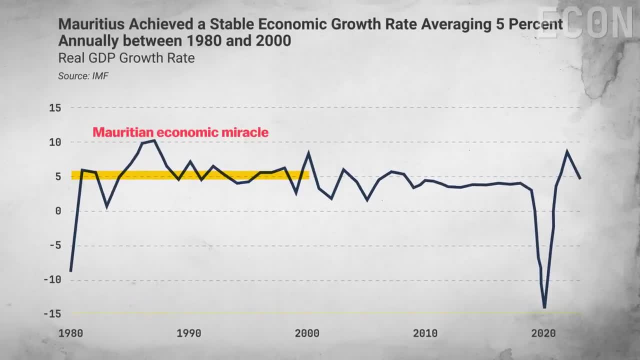 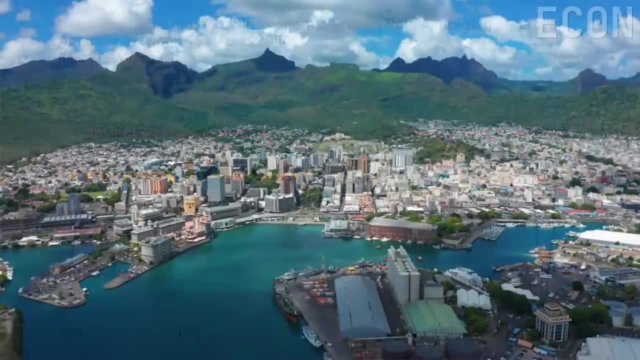 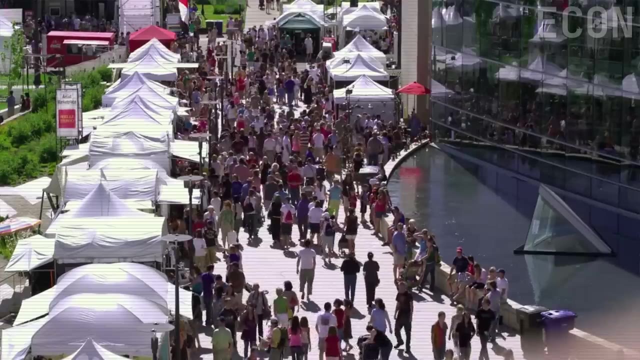 and 2000.. This period, often called the Mauritian Economic Miracle, has generally been attributed to the role of Foreign Direct Investment, or FDI, in transforming the country from a stagnant monocrop economy to one with sustainable growth and development. While having sensible economic policies is crucial, it's not enough. Several other 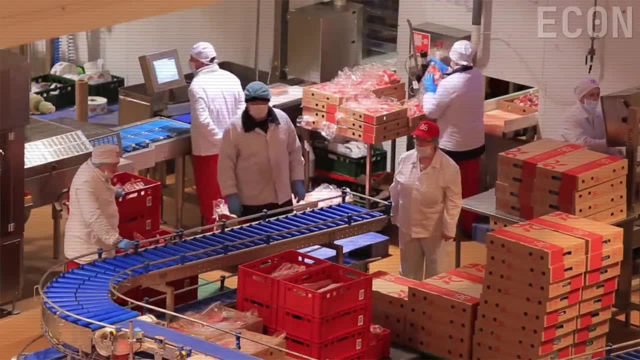 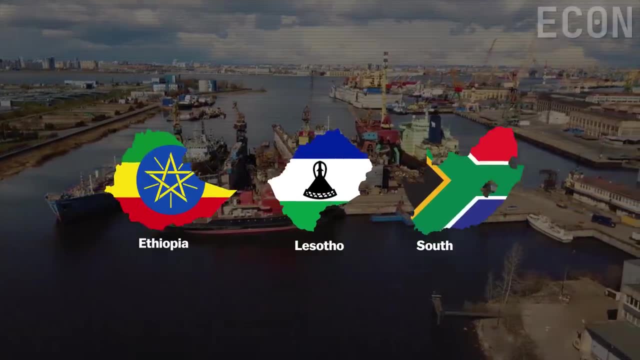 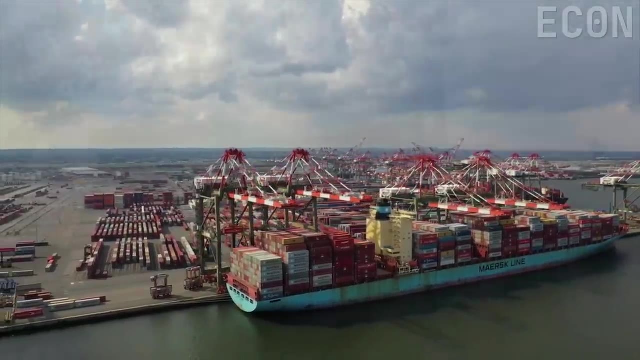 African countries also tried to boost manufacturing by attracting foreign investors to the island economy. Only a few, including Ethiopia, Lesotho and South Africa, succeeded. Trade and investment policies were just a portion of what contributed to Mauritius' success. Another critical element was the resilience of its institutions. 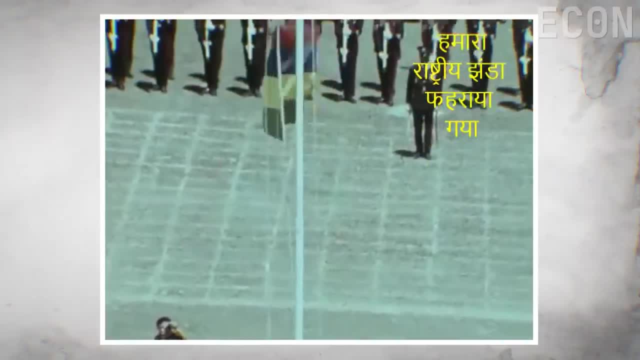 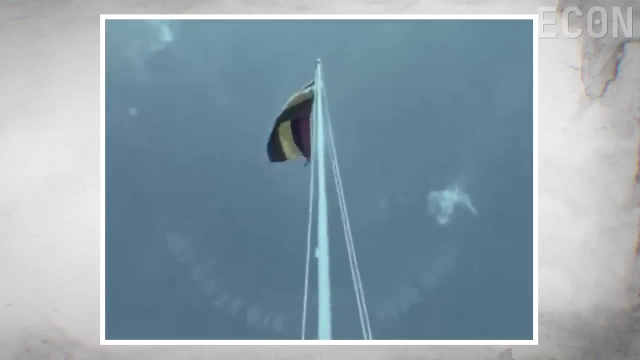 Ever since gaining independence, Mauritius has maintained peaceful elections, adhered to the rule of law, upheld integrity within its courts and managed to maintain a relatively low level of corruption. When we look at Mauritius' history, we can see that the island economy has been a major 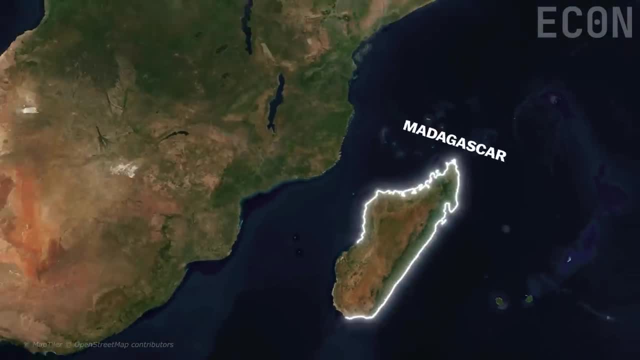 asset to Mauritius. In the 1970s, Mauritius was one of the world's largest exporters of foreign oil. In the 1970s, Mauritius was one of the world's largest exporters of foreign oil. When we look at Mauritius' biggest neighbour, Madagascar, its larger size and richer natural 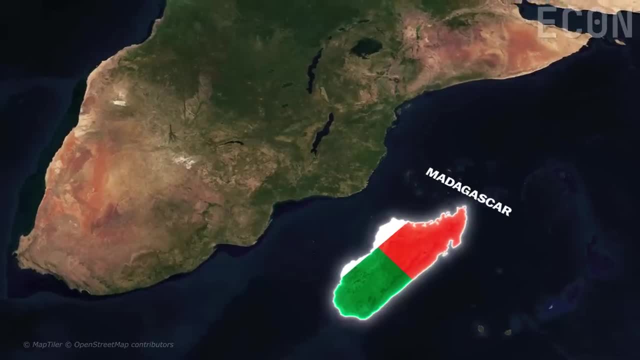 resources seemed to position it for potential success. However, this was not the case. In the 1970s, just as Mauritius started to attract foreign investors, Madagascar adopted a socialist approach marked by economic centralisation and state control. This decision led to the expulsion of investors and the nationalisation of two American oil. 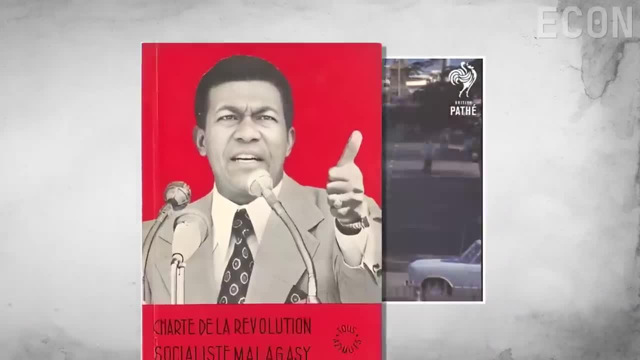 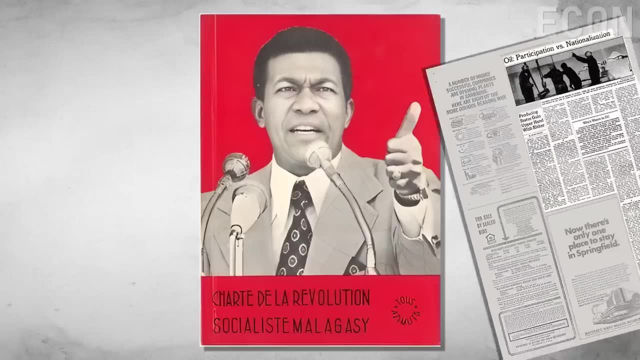 companies. While Mauritius worked to discover new export markets for the island economy, Mauritius was also a major investor in foreign oil. In the 1970s, Mauritius was a major investor in foreign oil. However, this decision led to the expulsion of investors and the nationalisation of two. 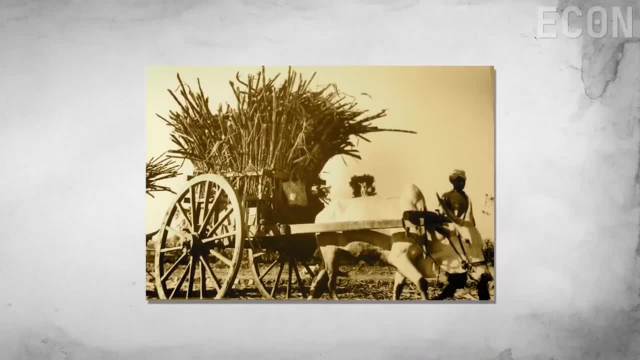 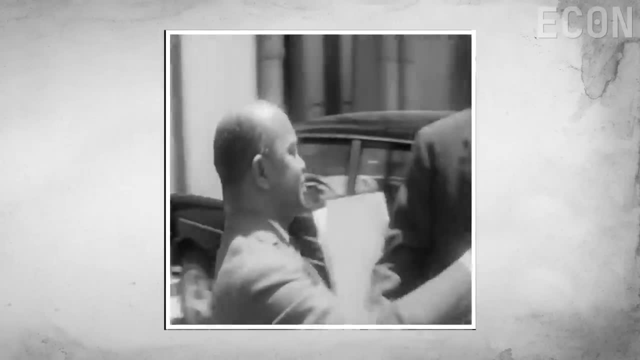 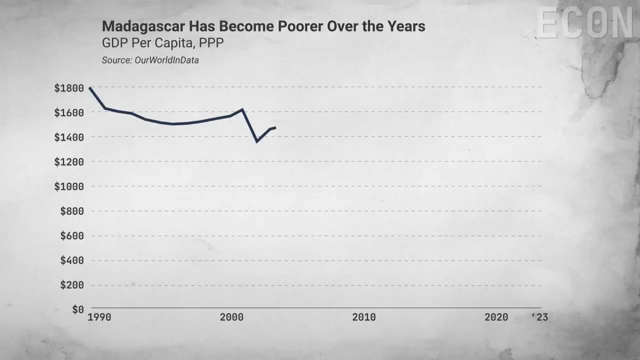 American oil companies. While Mauritius worked to discover new export markets for its sugar industry, Madagascar took a different path by seizing land from its commercial farmers. Unfortunately, the Malagasy economy suffered a severe collapse. Sirius In Graceland is one of the few countries to have become poorer over the years. 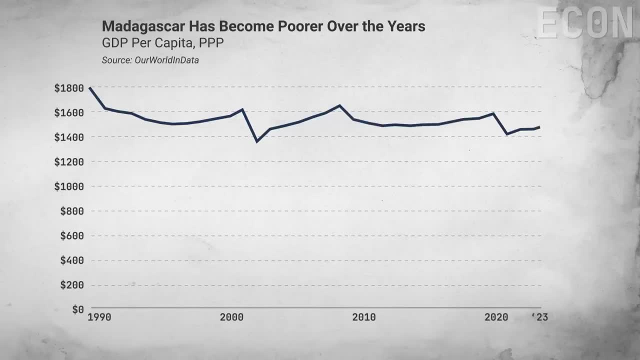 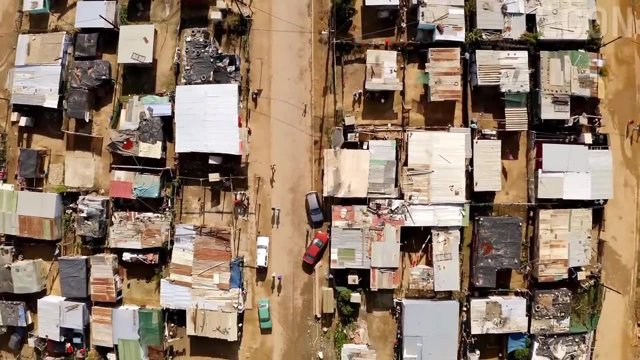 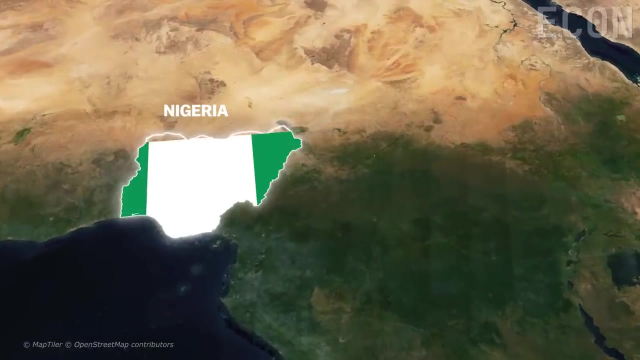 Because of disastrous socialist policies, ruralilOkay, the Malagasy economy suffered riots and generally chronic political instability. The main problem of the African economy is corruption and mismanagement. Power really corrupts. So too does a resource-rich economy like Nigeria's, the largest economy of Africa. 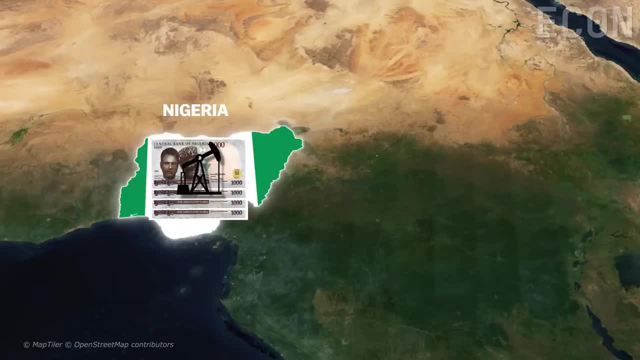 where easy access to oil revenues paves the way for unethical practices. The Transparency International Corruption Perception Index ranks Nigeria 150th out of 180 countries. According to The Economist, by the year 2030, the size of Africa's largest economy should. 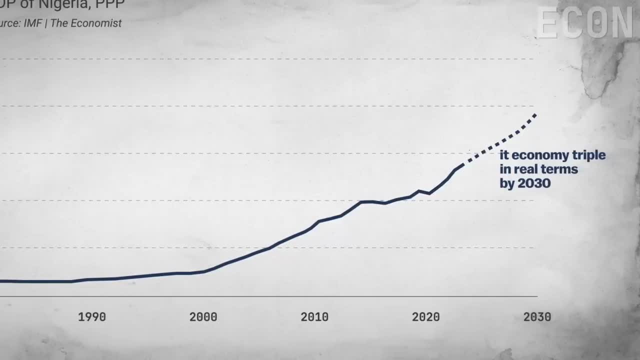 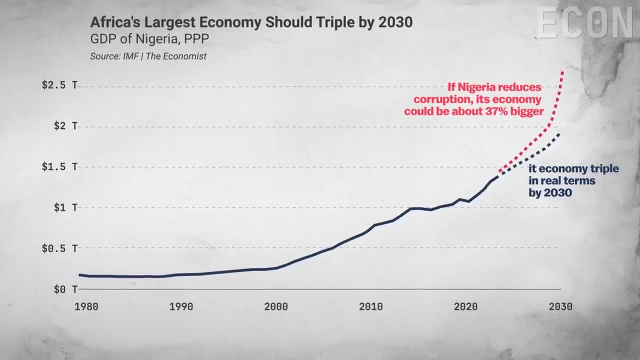 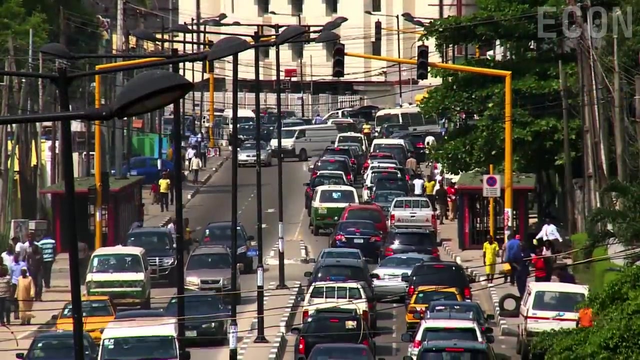 triple in real terms, And if Nigeria manages to reduce corruption levels comparable to Malaysia, its economy could be about 37% bigger. Nigeria has for long been regarded as the poster child for the curse of oil wealth, Yet despite this, Nigeria achieved strong economic growth for over a decade. in the 21st 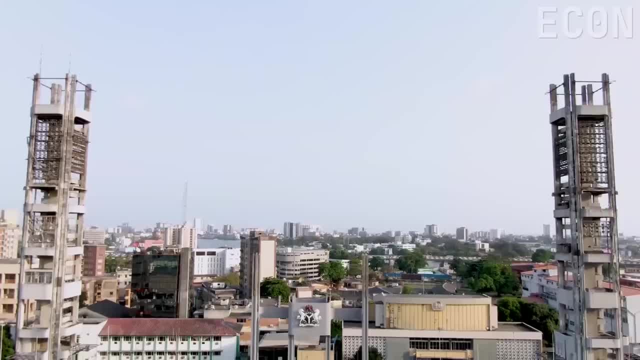 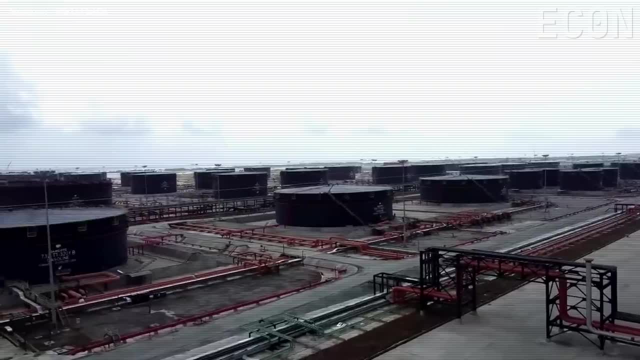 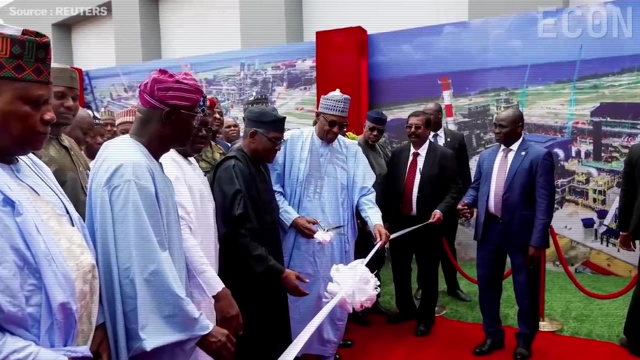 century, driven largely by policy reforms in non-oil sectors. Nigeria's major development challenge is not the oil curse, but rather one of achieving economic diversification beyond oil, subsistence agriculture, informal activities and across its sub-national entities. Its challenge of economic diversification is situated within the political setting of 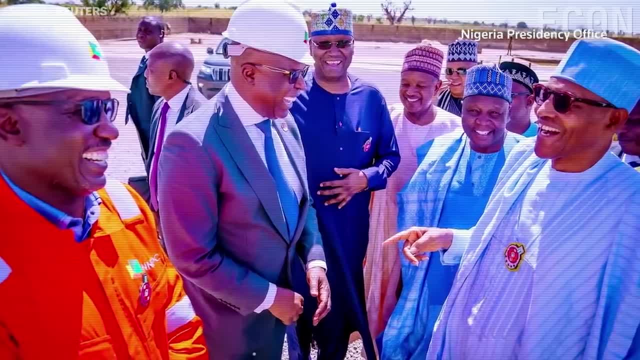 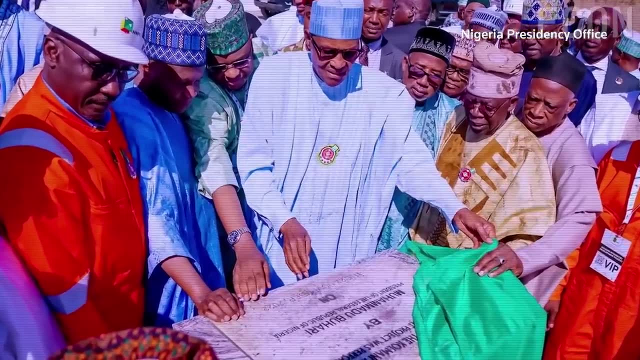 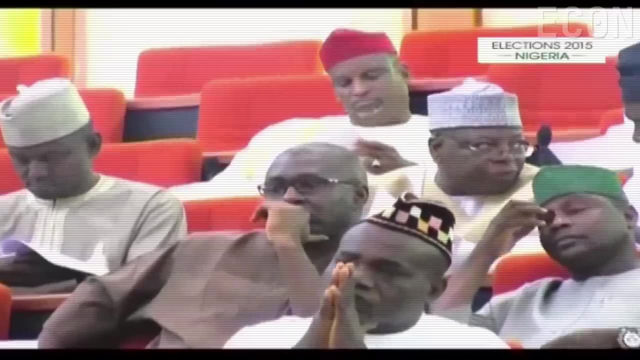 an unstable distribution of power among individual, group and institutional actors. Public institutions often hire the family and friends of the boss rather than the best candidates. In turn, those institutions become more inefficient and deliver less of what they are meant to, whether it is education or roads. 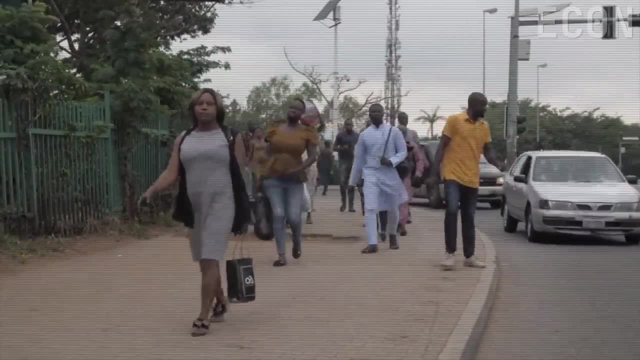 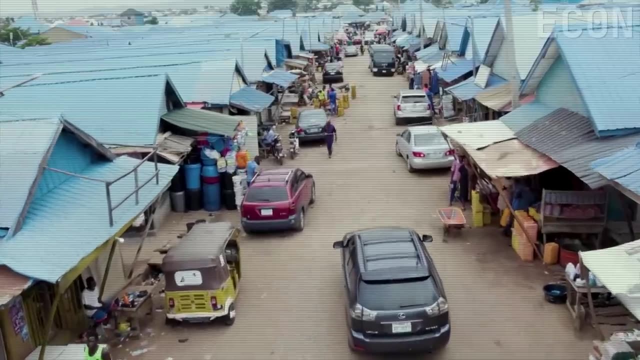 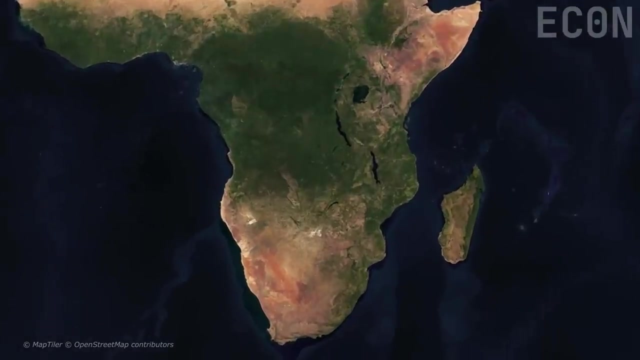 In addition, countries where corruption is high attract less foreign investment. They have higher prices and lower tax bases. Nigeria's tax-to-GDP ratio is only about 8%, compared with more than 25% in South Africa, Although South Africa, the economic powerhouse, is not immune to corruption and mismanagement. 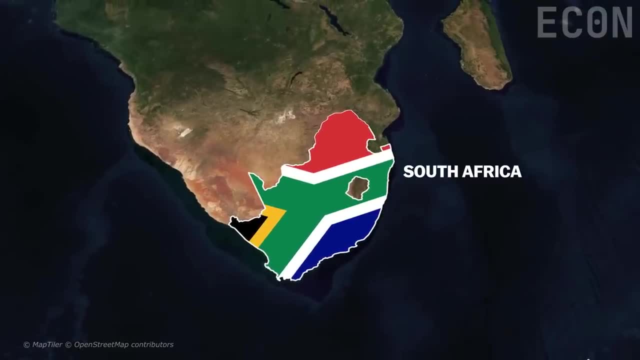 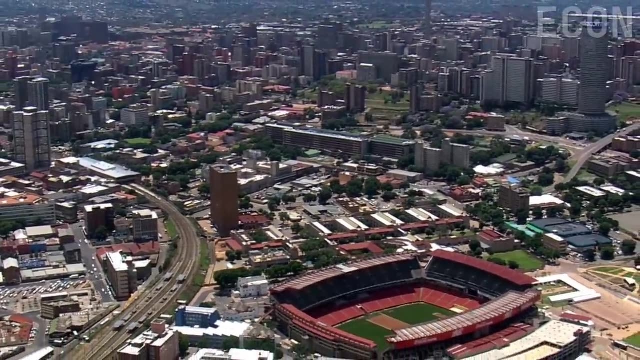 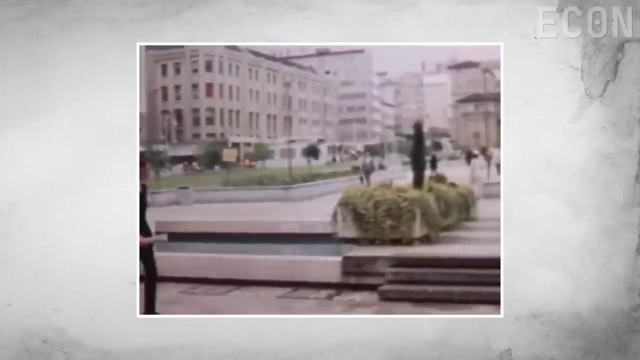 it has succeeded. It has successfully diversified its economy, with a growing and sizeable middle class. The economy of South Africa is the second-largest in Africa and the most industrialised, technologically advanced and diversified economy in Africa. For the first 15 years of democracy, South Africa enjoyed the advantages of both effective institutions and a shared willingness of stakeholders to believe in the power of cooperation. This enabled the country to move beyond counter-productive conflict and pursue win-win outcomes. Growth began to accelerate, which created new opportunities for expanding the middle class. Increased fiscal space made it possible to broaden access to public services and to social 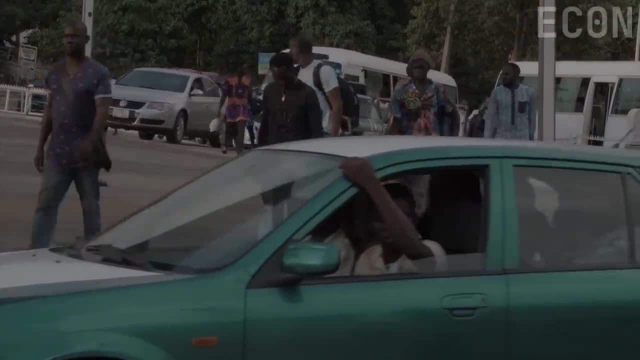 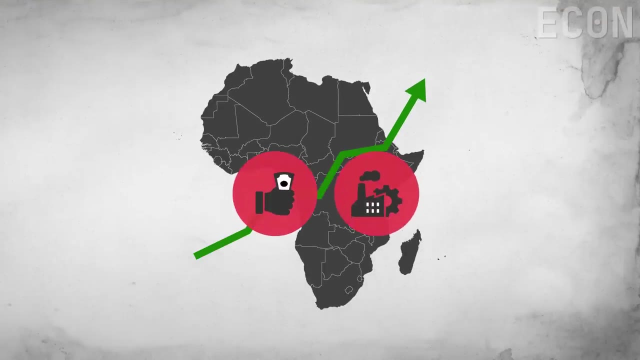 grants which reduced absolute poverty. There is no doubt Africa is growing and its growth is already being driven by internal consumption and investment. The expansion of regional trade would reinforce that dynamic, especially in industry. Manufactured goods make up only 19% of African wealth. 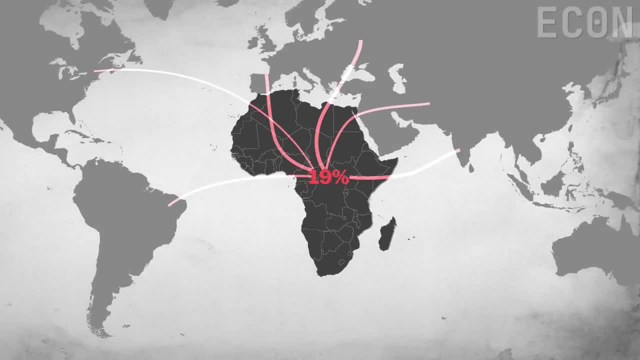 The economy of South Africa is growing, and its growth is already being driven by internal consumption and investment. As of the end of the 20th century, the world's most important export sector- the oil and gas sector- is a global market. As of the end of the 20th century. the world's most important export sector, the oil and gas sector, is a global market. The country has the highest exports to the rest of the world, but 43% of what they sell. 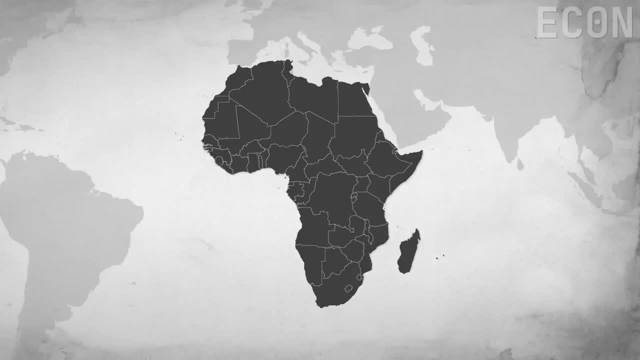 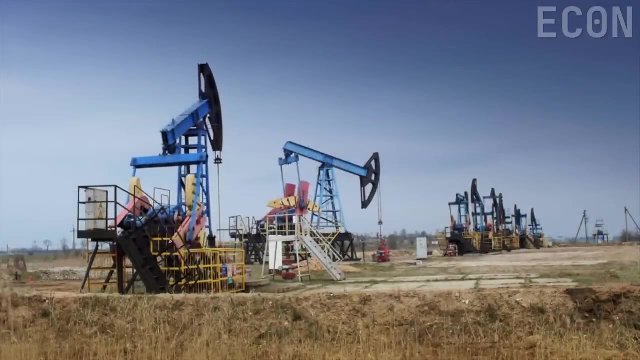 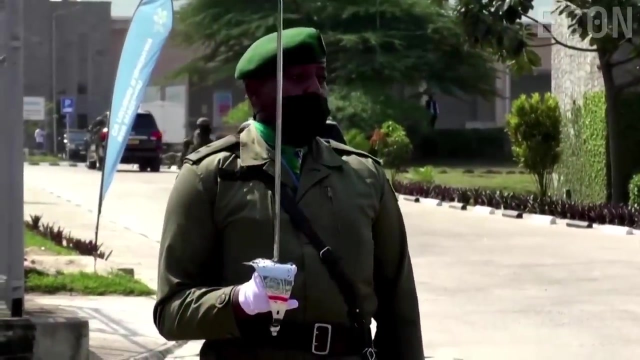 to each other. To access larger markets, companies must engage in global exports. As they adapt to global competition, their productivity also improves. Nigeria is gradually reducing its reliance on oil exports. Rwanda is becoming a hub for conferences, attracting upscale tourists and thriving business. 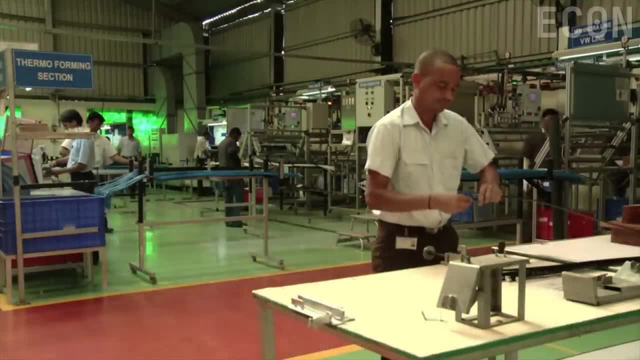 services firms. Lesotho and Ethiopia are building factories and an Asian-style manufacturing. As of the end of the 20th century, the oil sector has grown. It is a growing market. It is becoming a hub for conferences, attracting upscale tourists and thriving business services. 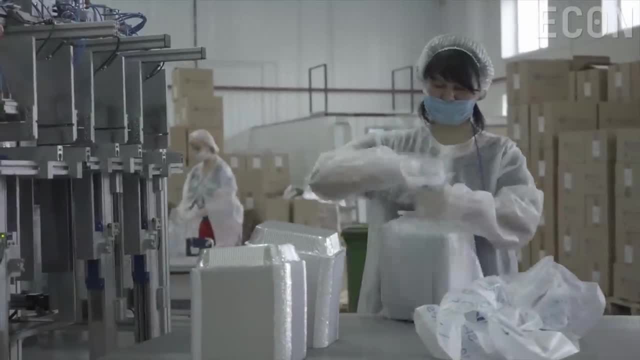 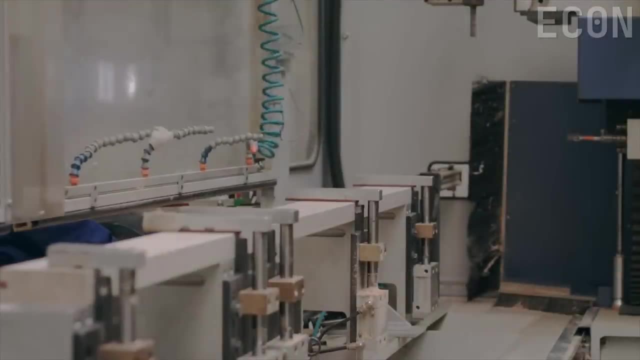 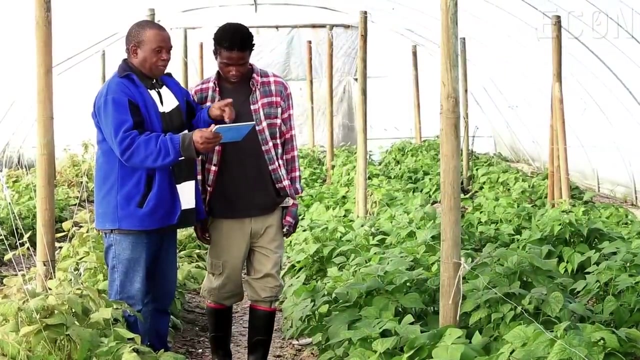 manufacturing hub. Some economists argue that automation, competition and shifting demand are limiting the prospects for countries seeking to replicate Asia's economic miracle. Yet not everyone needs a factory job. Many Africans will move from subsistence farms to commercial ones, or from living alongside a game reserve to guiding tourists around one. 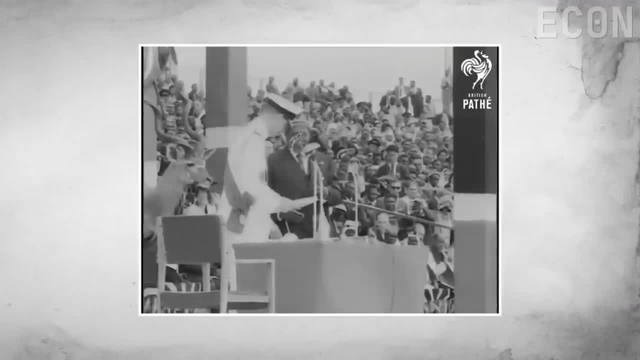 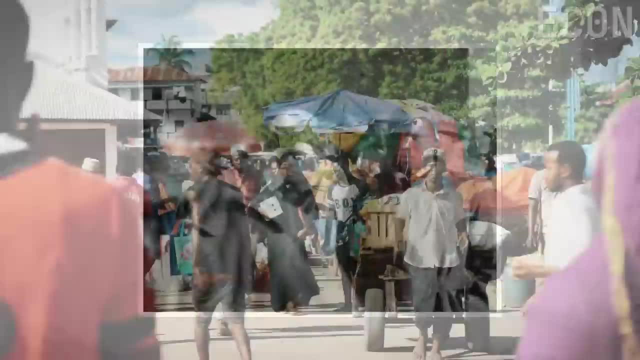 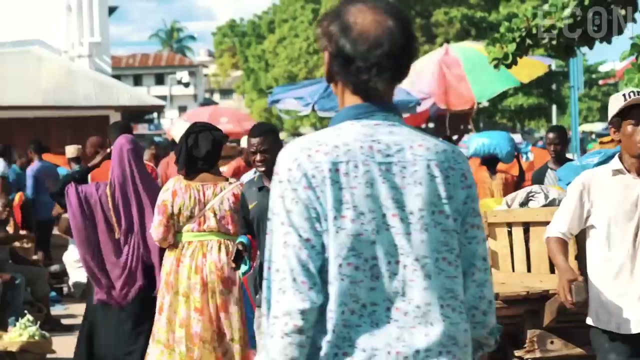 Since colonial powers carved up Africa, the continent's population numbered fewer than 100 million people, which accounted for approximately one-third of Europe's population at the time. Today, there are almost two Africans for every European. Some outsiders see this rapid population growth as a potential recipe for disaster. 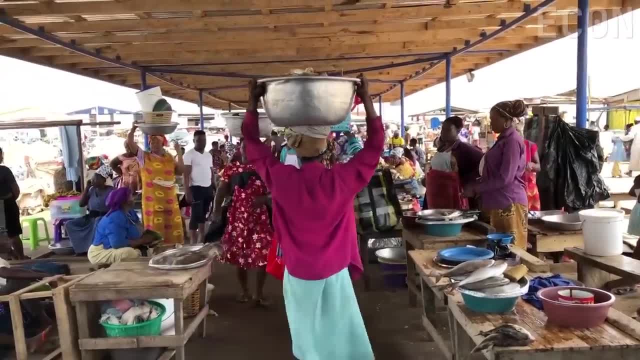 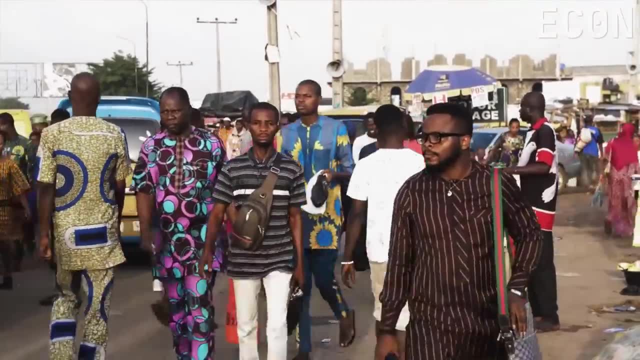 Although the poverty rate is falling, about a third of children are still malnourished. Every month, about one million Africans enter the job market. Many of them do not have the education or skills they need. More than a third of African children do. 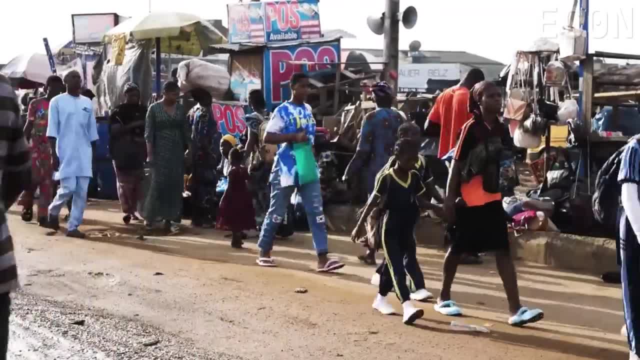 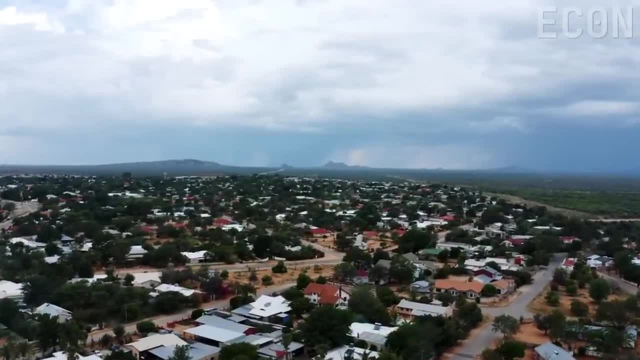 not have the education or skills they need. In Mozambique and Madagascar, that rate jumps to more than half Over the longer term. the major trends taking hold – rapid urbanisation, increasing migration and remittances, a rising share of children in school. 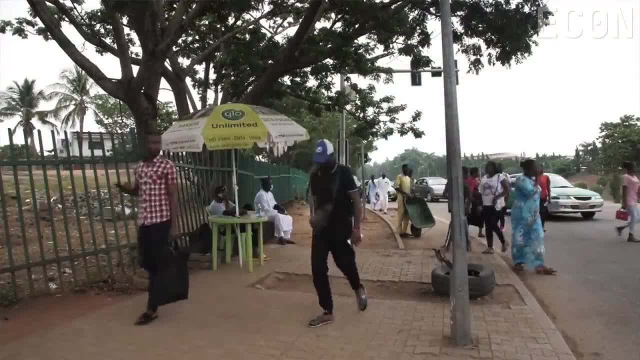 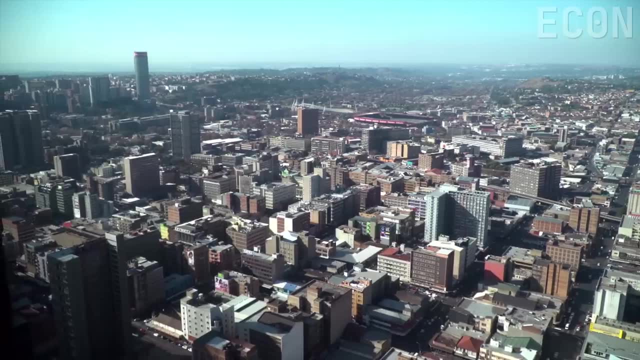 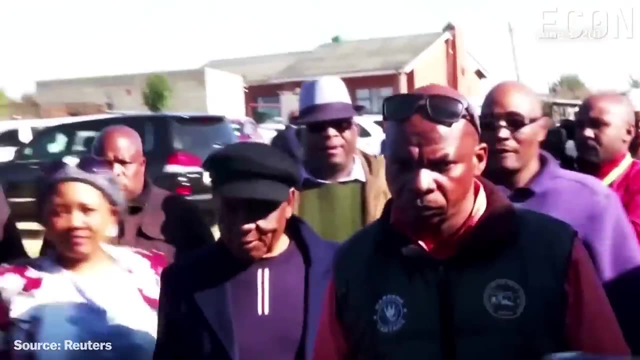 the hundreds of thousands of students at universities abroad – are reasons for hope. These trends provide reasons for optimism. The most crucial lesson, and one that holds the most promise, is that many of these trends reinforce one another. Countries with more capable bureaucracies and open democratic systems tend to fare better. 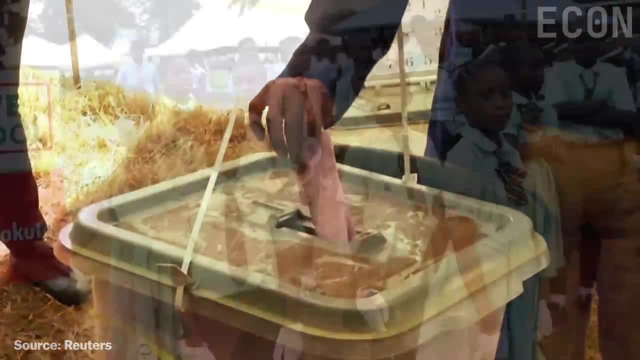 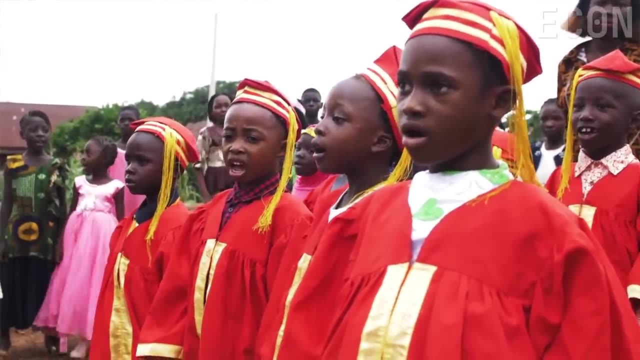 economically and invest more in education. Strengthened economies and improved education in turn contribute to decelerating population growth and enhancing dependency ratios. While not all nations are part of this virtuous cycle, the differences are stark for those that are.